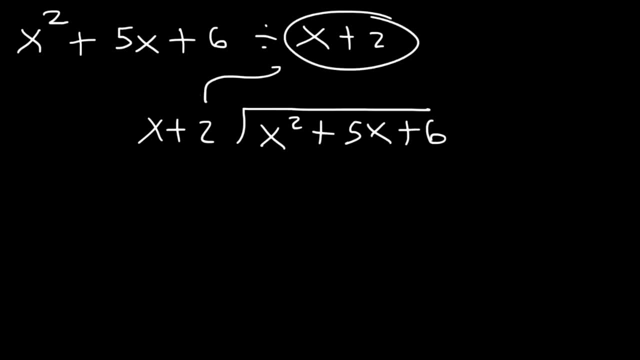 The denominator should go on the outside. So the first thing we need to do is divide. x squared divided by x is equal to 1.. x squared divided by x is basically x. What we need to do is subtract the exponents: 2 minus 1 is equal to 1.. Now, after you divide, the next step is to multiply. 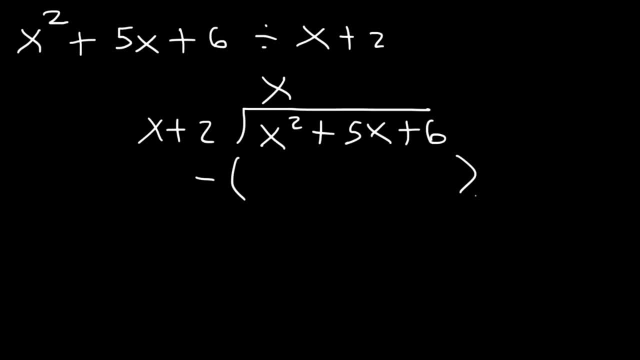 Let's put a negative sign and parentheses. Everything that's going to be written here. we need to distribute by a negative sign or basically just change a sign. If we multiply x by x, that is equal to x squared, And if we multiply x by positive 2,. 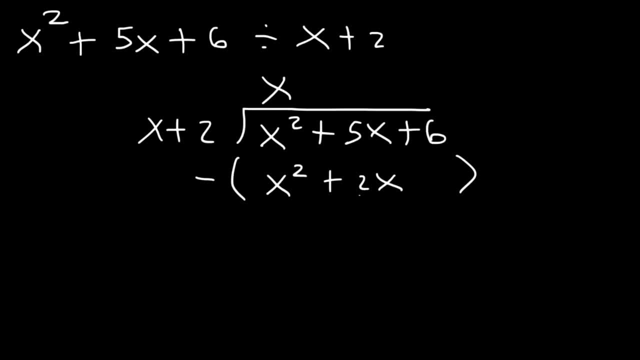 that's equal to positive 2x. At this point, subtract x squared minus x squared, Those two will cancel and it's equal to 0.. Next, 5x minus 2x is equal to positive 3x. 6 minus nothing is basically equal to 6.. So you could bring down the 6.. 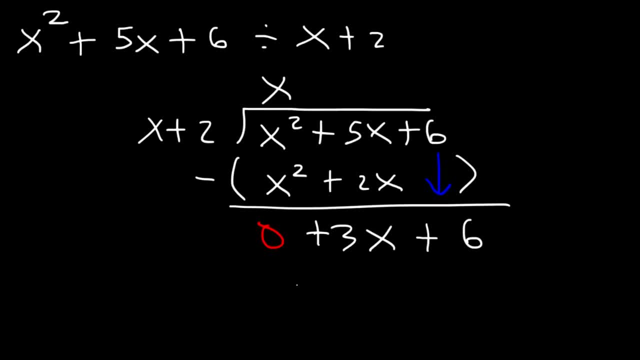 Now the next thing that we need to do is divide. We're going to follow the same three steps as we did before. We're going to divide, multiply and subtract 3x. divided by x, that's equal to positive 3.. And then now we're going to multiply 3 times. x is 3x. 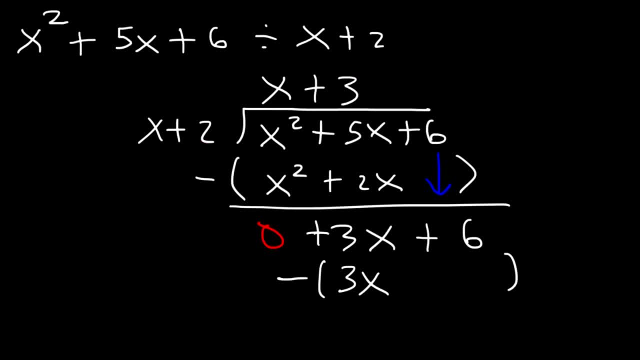 And then 3 times 2, that's equal to positive 6.. So now we could subtract: 3x minus 3x is 0.. 6 minus 6 is 0. So the remainder is 0.. Therefore, the solution is what we see here. 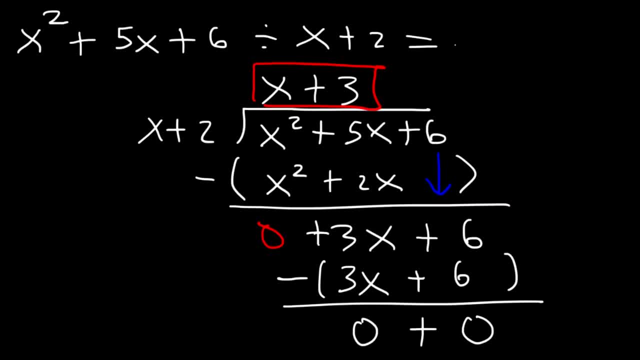 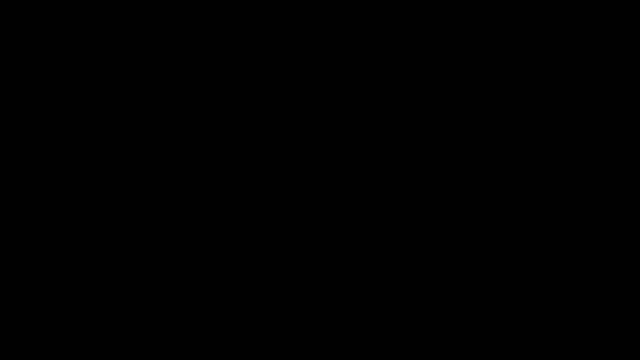 x squared plus 5x plus 6, divided by x plus 2, that's equal to x plus 3.. So that's the answer. Now let's work on another example. Try this one: Divide 2x cubed plus 8x squared minus 6x plus 10.. Go ahead and 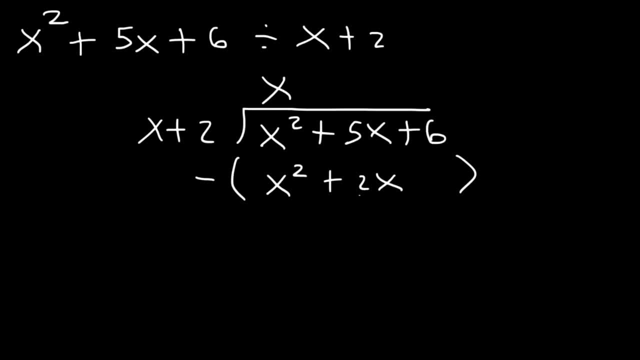 that's equal to positive 2x. At this point, subtract x squared minus x squared, Those two will cancel and it's equal to 0.. Next, 5x minus 2x is equal to positive 3x. 6 minus nothing is basically equal to 6.. So you could bring down the 6.. 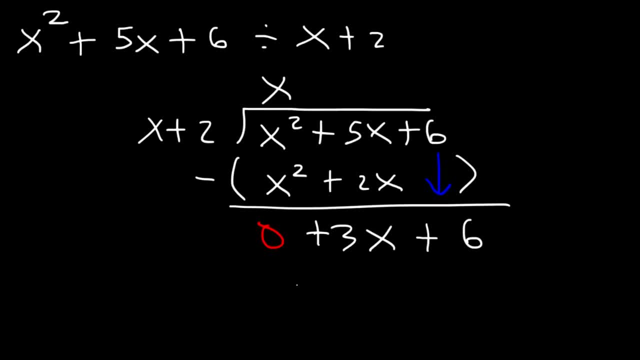 Now the next thing that we need to do is divide. We're going to follow the same three steps as we did before. We're going to divide, multiply and subtract 3x. divided by x, that's equal to positive 3.. And then now we're going to multiply 3 times. x is 3x. 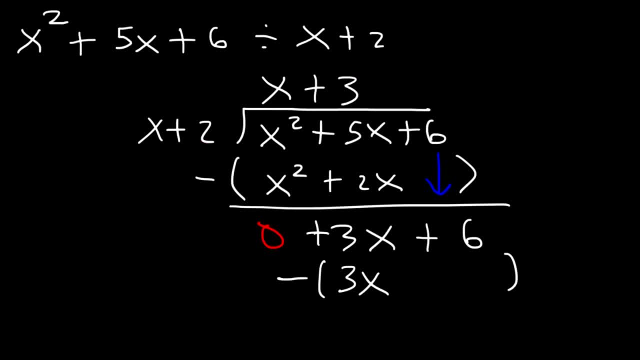 And then 3 times 2, that's equal to positive 6.. So now we could subtract: 3x minus 3x is 0.. 6 minus 6 is 0. So the remainder is 0.. Therefore, the solution is what we see here. 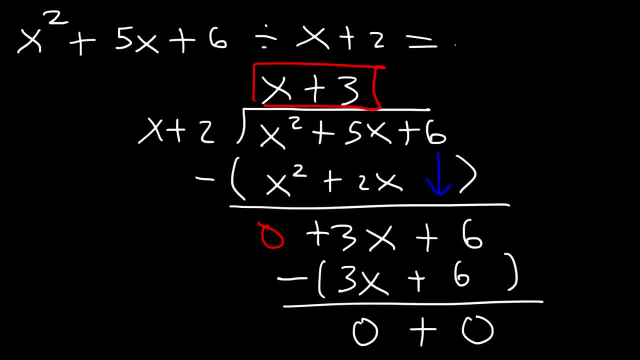 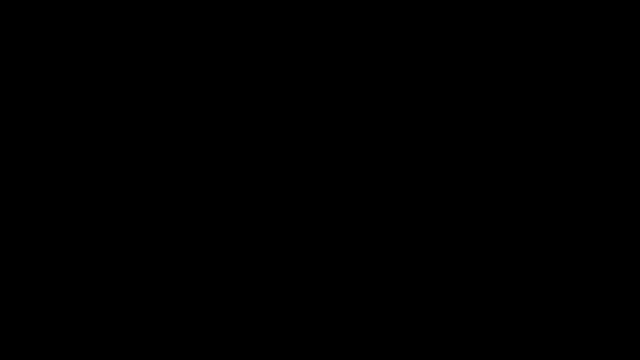 x squared plus 5x plus 6, divided by x plus 2, that's equal to x plus 3.. So that's the answer. Now let's work on another example. Try this one: Divide 2x cubed plus 8x squared minus 6x plus 10.. Go ahead and 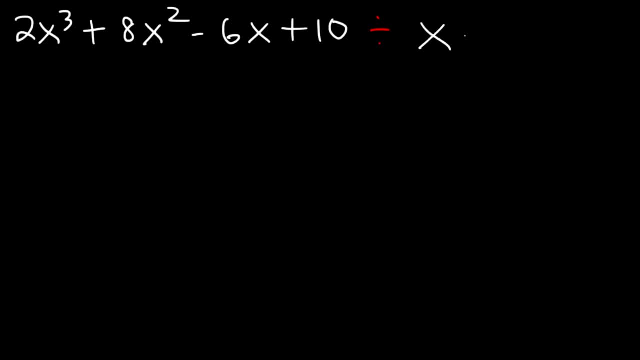 divided by x minus 2.. So feel free to pause the video and work on this example. So first, let's write it out. Now, the first thing we're going to do is we're going to divide. Let's divide 2x cubed by x. 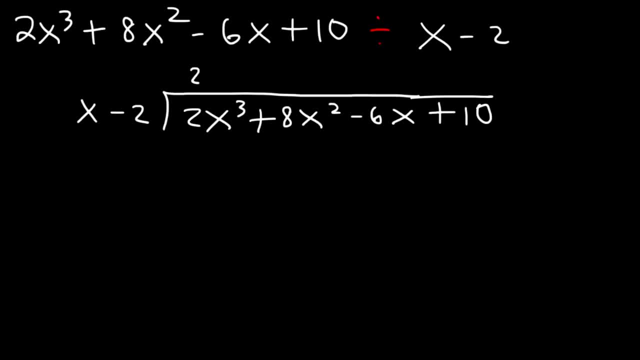 So that is equal to 2x squared. Next, let's multiply 2x squared times x. that's equal to 2x cubed. The first one's always going to be the same. These two should always match. And then 2x squared times negative 2, that's equal to negative 4x squared. 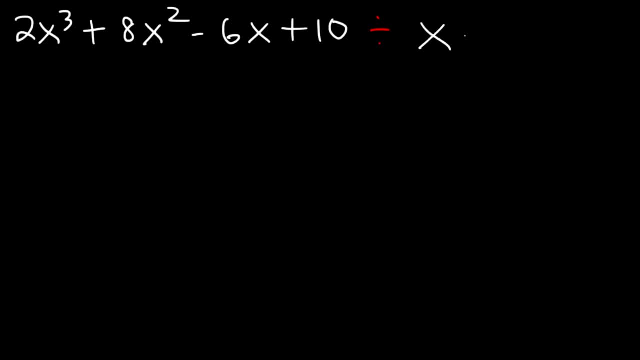 divided by x minus 2.. So feel free to pause the video and work on this example. So first, let's write it out. Now, the first thing we're going to do is we're going to divide. Let's divide 2x cubed by x. 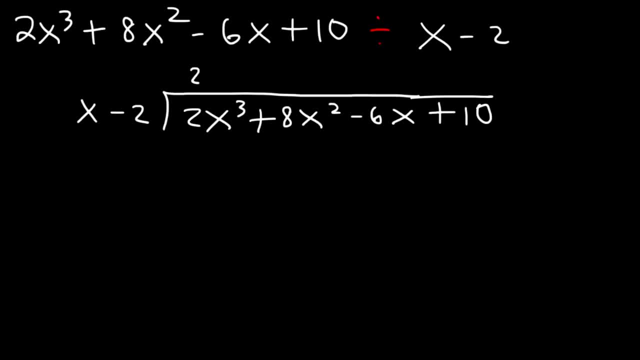 So that is equal to 2x squared. Next, let's multiply 2x squared times x. that's equal to 2x cubed. The first one's always going to be the same. These two should always match. And then 2x squared times negative 2, that's equal to negative 4x squared. 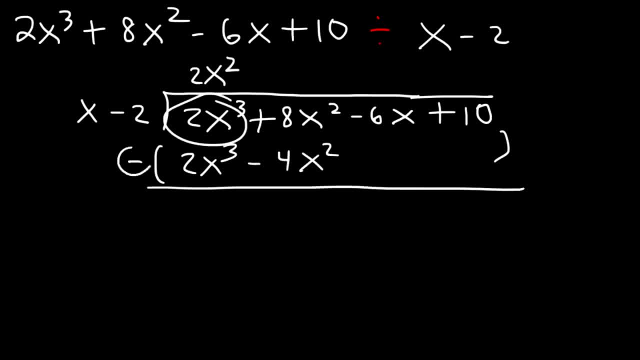 So now let's subtract 2x squared times x, that's equal to negative 4x squared. 2x cubed minus 2x cubed. those two will always cancel, And so that's 0.. 8x squared minus negative 4x squared is basically the same as 8x squared plus 4x squared. 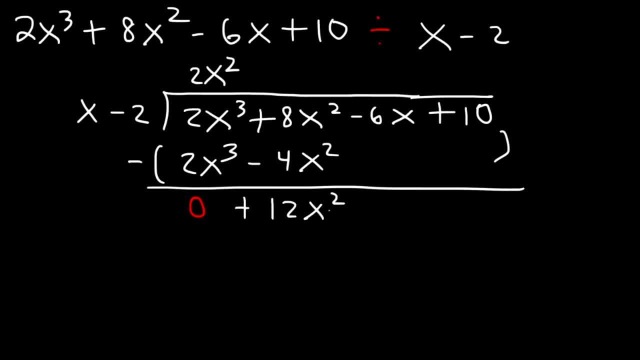 And that's equal to positive 12x squared. Now everything else, we're just going to bring it down to the next level. So we have negative 6x and positive 10.. Now let's repeat these three steps: Divide, multiply and subtract. 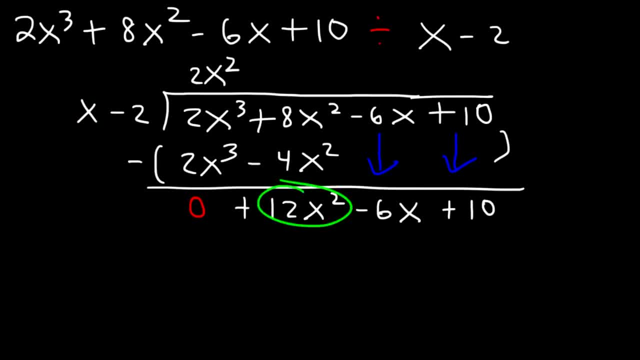 So let's divide 12x squared by x, So that's equal to positive 12x. Now let's multiply 12x times x, that's 12x squared, And 12x times negative 2, that's equal to negative 24x. 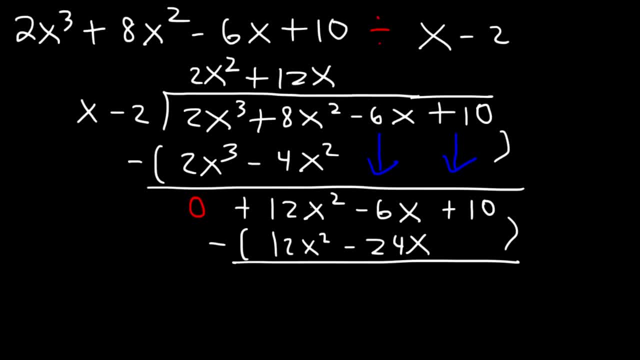 Now let's subtract. Let's subtract So we have 12x squared minus 12x squared, which is equal to 0.. And negative 6x minus negative 24x, which is the same as negative 6x plus 24x. 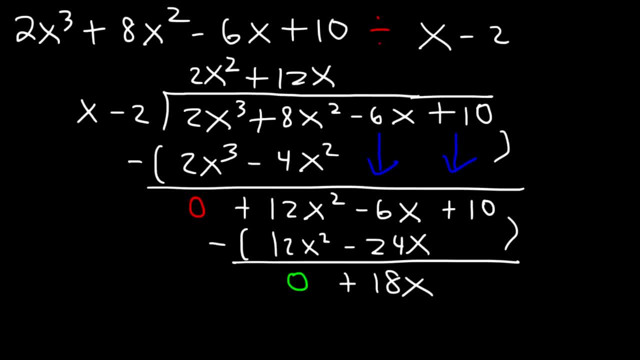 That's positive 18x. And now let's bring it down to 10.. So we have 18x plus 10.. So now let's divide 18x. divided by x is positive 18.. And then multiply 18 times x is 18x. 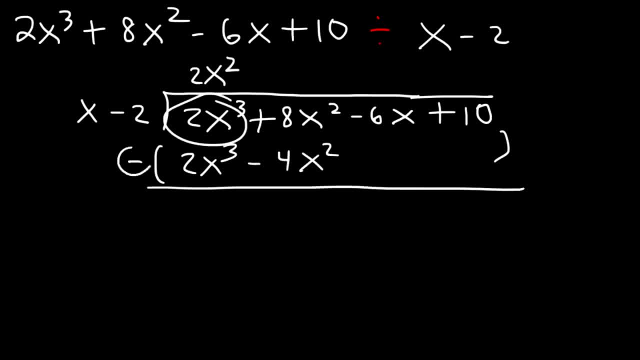 So now let's subtract 2x squared times x, that's equal to negative 4x squared. 2x cubed minus 2x cubed. those two will always cancel, And so that's 0.. 8x squared minus negative 4x squared is basically the same as 8x squared plus 4x squared. 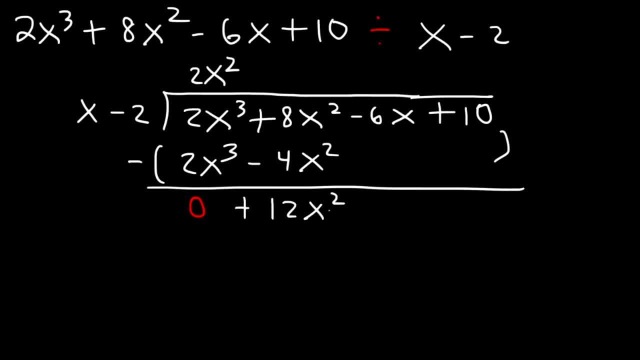 And that's equal to positive 12x squared. Now everything else, we're just going to bring it down to the next level. So we have negative 6x and positive 10.. Now let's repeat these three steps: Divide, multiply and subtract. 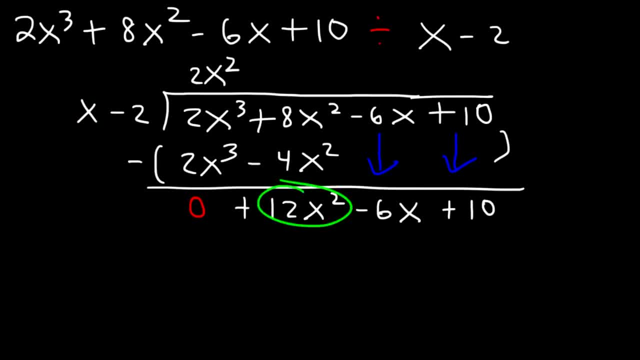 So let's divide 12x squared by x, So that's equal to positive 12x. Now let's multiply 12x times x, that's 12x squared, And 12x times negative 2, that's equal to negative 24x. 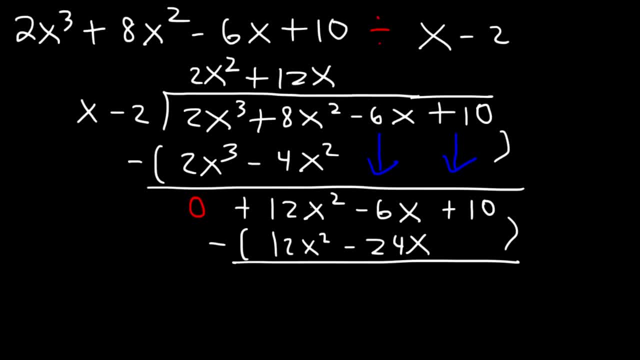 Now let's subtract. Let's subtract, So we have 12x squared. 12x squared minus 12x squared, which is equal to 0.. And negative 6x minus negative 24x, which is the same as negative 6x plus 24x. 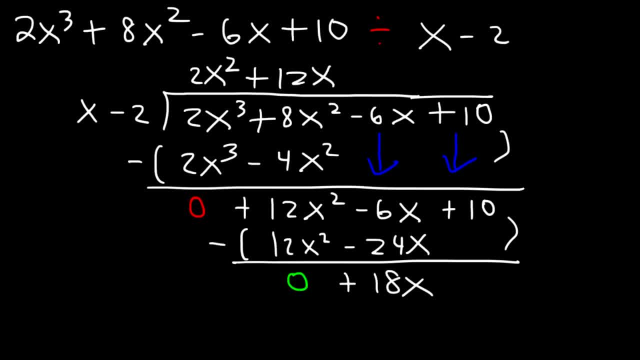 That's positive 18x. And now let's bring down the 10. So we have 18x plus 10.. So now let's divide: 18x divided by x is positive 18.. 18x divided by x is positive 18.. 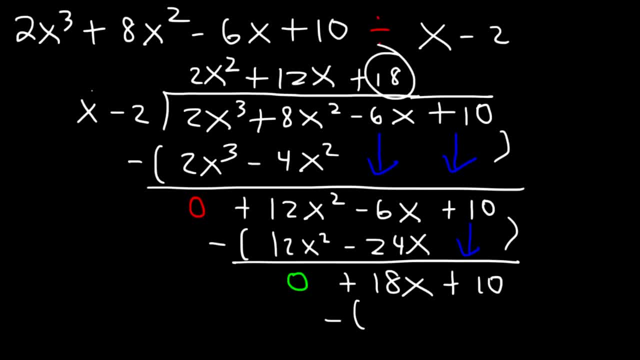 And then multiply 18 times x is 18x, And 18 times negative 2,, that's negative 36.. So now let's subtract: 18 minus 18 is 0. And 10 minus negative 36, we have two negative signs. 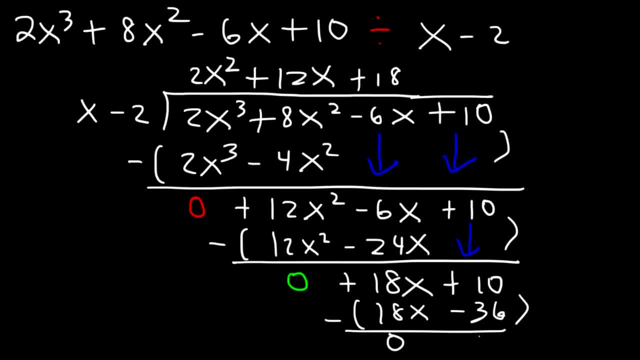 That's the same as 10 plus 36.. 10 plus 36 is 46. Now we can't divide 46 by x, So the remainder is 46. So how do we write the answer whenever we have a remainder? So it's going to be what you see here plus the remainder, which is 46,. 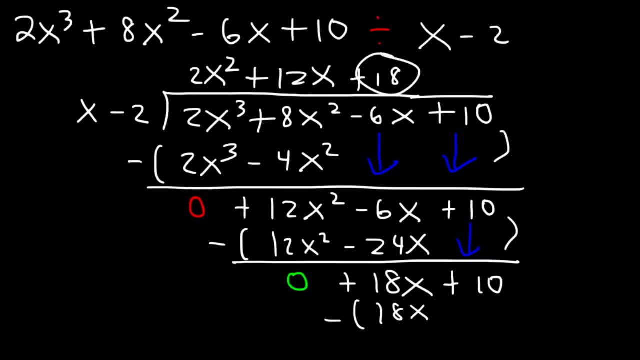 And 18 times negative 2, that's negative 36.. So now let's subtract: 18 minus 18 is 0. And 10 minus negative 36, we have two negative signs. That's the same as 10 plus 36.. 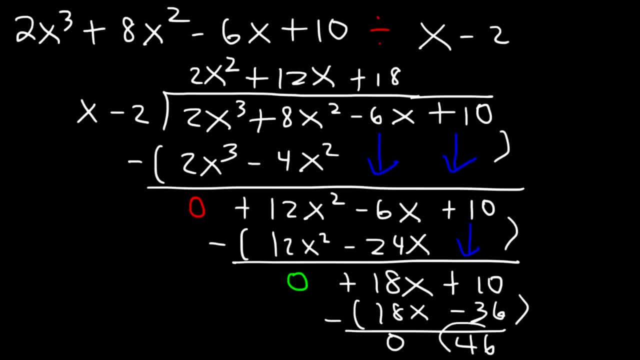 10 plus 36 is 46. Now we can't divide 46 by x, So the remainder is 46. So how do we write the answer whenever we have a remainder? So it's going to be what you see here plus the remainder, which is 46,. 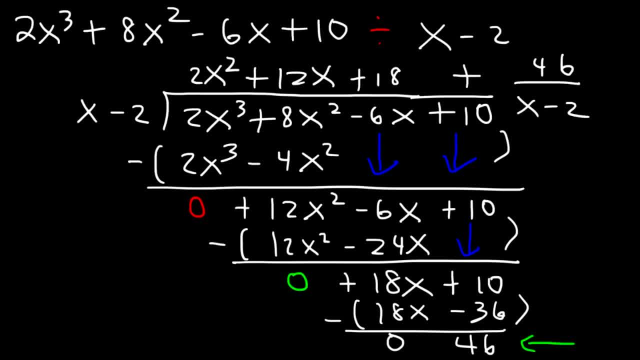 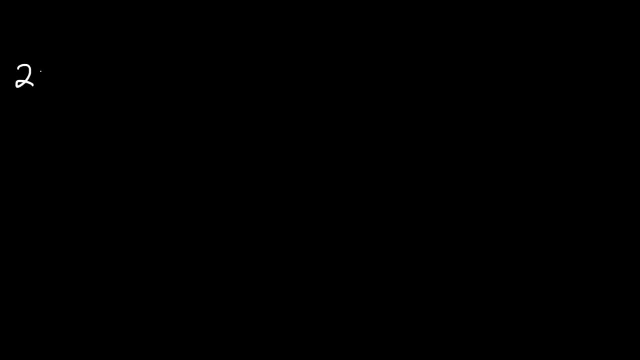 divided by what you tried to divide it by, which is x minus 2.. So, therefore, the final answer is: 2x squared plus 12x plus 18 plus 46, divided by x minus 2.. So all of that is equal to 2x cubed plus 8x squared minus 6x plus 10, divided by x minus 2.. 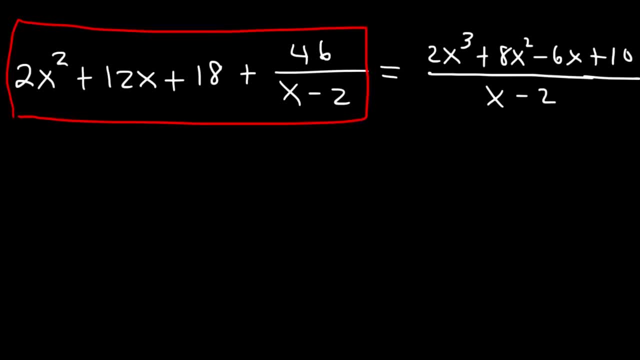 So this is the answer. Now let's move on to our next problem. Go ahead and divide 6x to the 4th, minus 9x squared plus 18, divided by x minus 3.. So take a minute, pause the video and work on this problem. 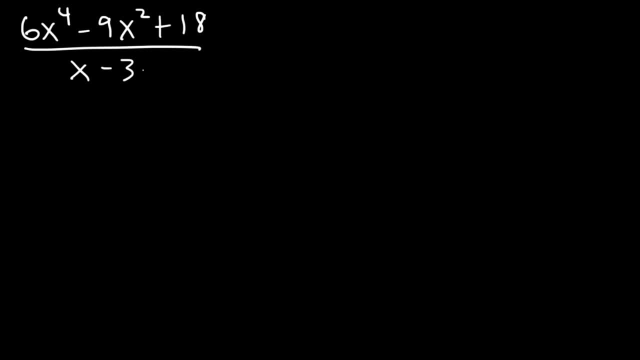 And once you have the solution, unpause it to see if you have the right answer And be careful with this one. So let's put the x minus 3 on the x And let's put the numerator on the inside. Now we need to put it in standard order. 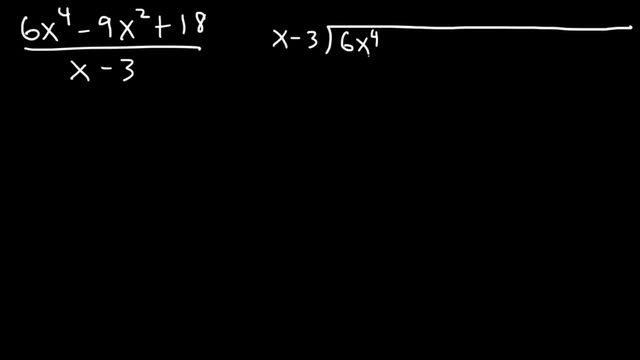 It's 6x to the 4th. Now we can't forget about the 0x cubed. So plus 0x cubed And then minus 9x squared, And don't forget about the 0x, And finally plus 18.. 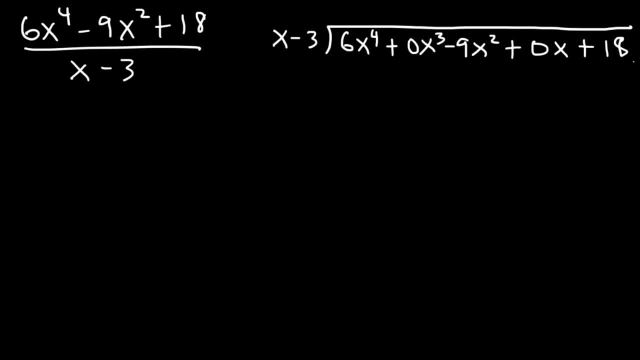 So we're going to follow the same three steps: Divide, multiply, subtract. So let's divide 6x to the 4th by x, So that's equal to 6x cubed. Simply subtract the 4 by 1, and you'll get the exponent 3.. 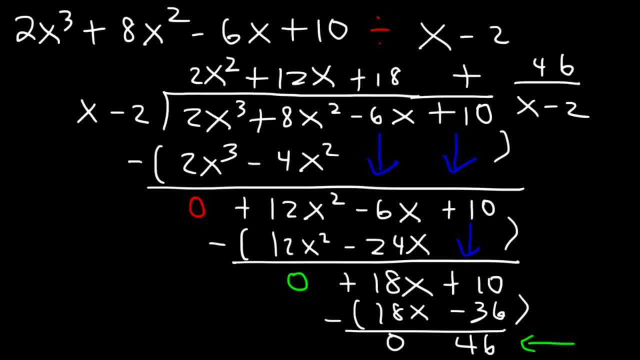 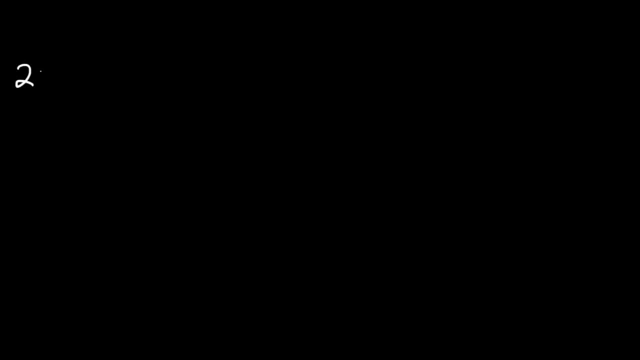 divided by what you tried to divide it by, which is x minus 2.. So, therefore, the final answer is 2x squared plus 12x, 12x plus 18 plus 46, divided by x minus 2.. So all of that is equal to 2x cubed plus 8x squared minus 6x plus 10, divided by x minus 2.. 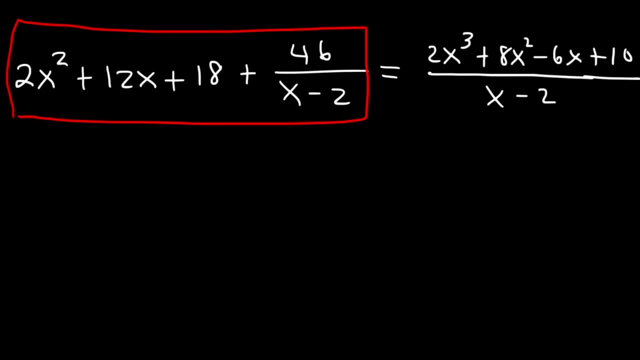 So this is the answer. Now let's move on to our next problem. Go ahead and divide 6x to the 4th, minus 9x squared plus 18 divided by x minus 3.. So take a minute, pause the video and work on this problem. 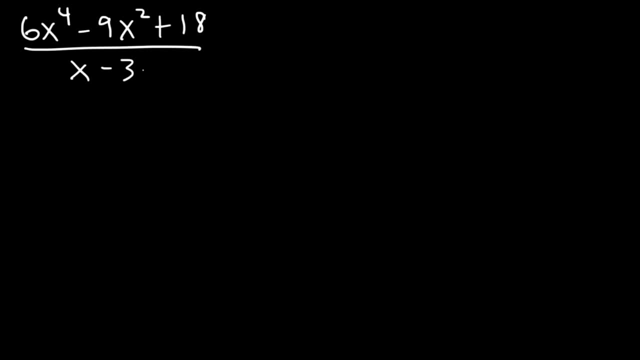 And once you have the solution, unpause it to see if you have the right answer And be careful with this one. So let's put the x minus 3 on the outside And let's put the numerator on the inside. Now we need to put it in standard order. 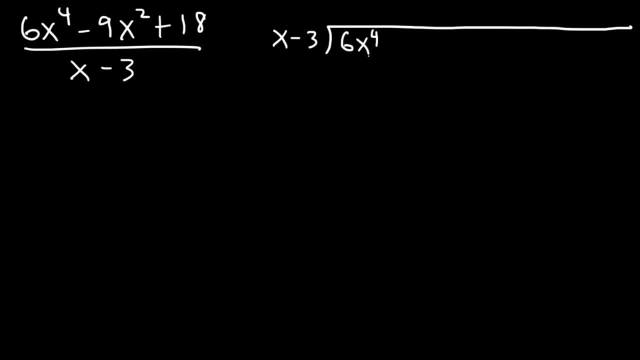 It's 6x to the 4th. Now we can't forget about the 0x cubed. So plus 0x cubed And then minus 9x squared, And don't forget about the 0x, And finally plus 18.. 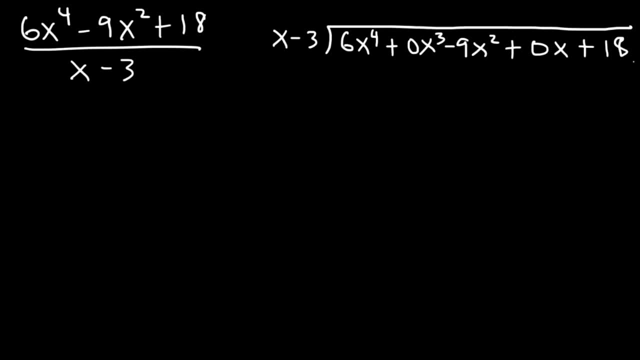 So we're going to follow the same three steps: Divide, multiply, subtract. So let's divide 6x to the 4th by x, So that's equal to 6x cubed. Simply subtract the 4 by 1, and you'll get the exponent 3.. 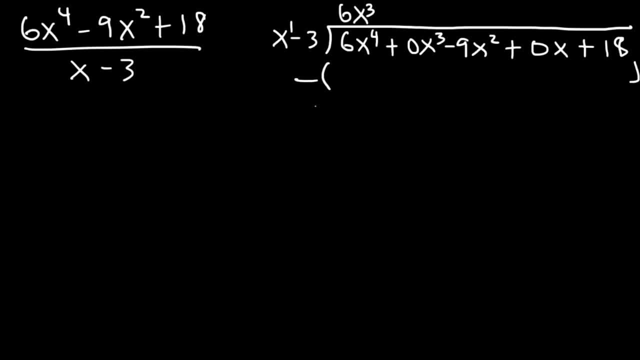 Now let's multiply 6x cubed times x, That's 6x to the 4th, And then we have 6x cubed times negative 3, which is negative 18x cubed. So at this point we need to subtract. 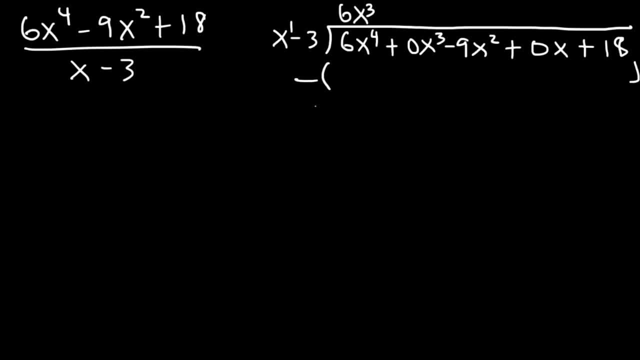 Now let's multiply 6x cubed times x, That's 6x to the 4th, And then we have 6x cubed times negative 3, which is negative 18x cubed. So at this point we need to subtract. 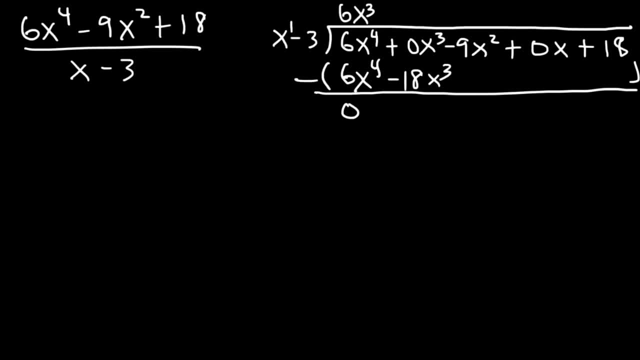 6x to the 4th, minus itself will be 0.. Now, 0x cubed minus negative 18x cubed. That's going to be just positive 8x. That's going to be negative 18x cubed. 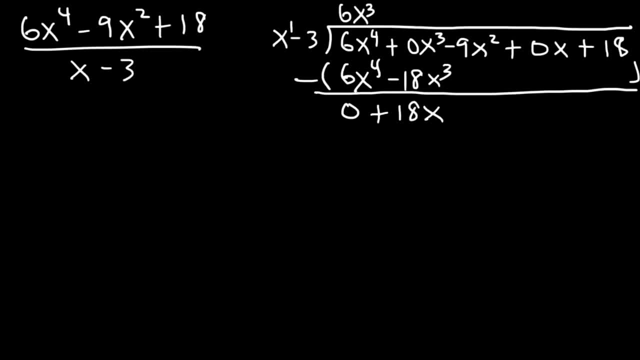 And everything else. we could bring it down so we can work on it in the next step. We really don't have to bring down everything. All we need really is just the next term, So we don't have to write the other two terms. 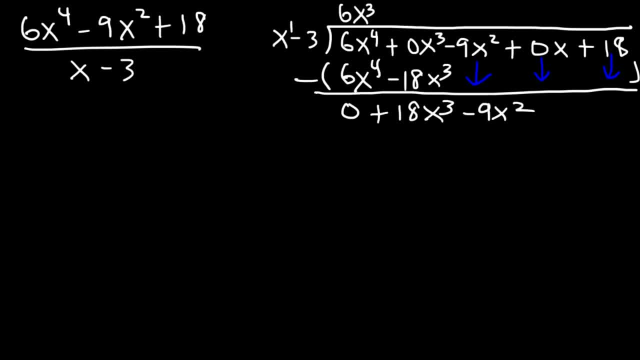 We can just focus on these two for now, But if you want to, you can write down the rest. Now let's divide 18x cubed by x. That's going to be negative 18x cubed. That's going to be negative 18x cubed. 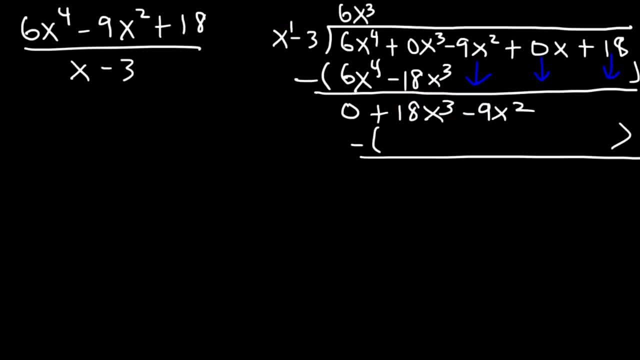 That's going to be negative 18x cubed. So that's going to be 18x squared. And now let's multiply 18x squared times x, That's 18x cubed. And then, if we multiply 18x squared by negative 3, that's negative 54x squared. 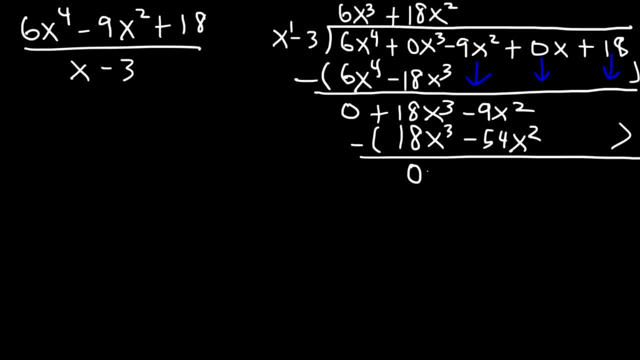 So this is going to be 0.. Negative 9. Minus That's negative 54. That's negative 9 plus 54. And 54 minus 9 is basically 65.. I take that back: It's not 65.. 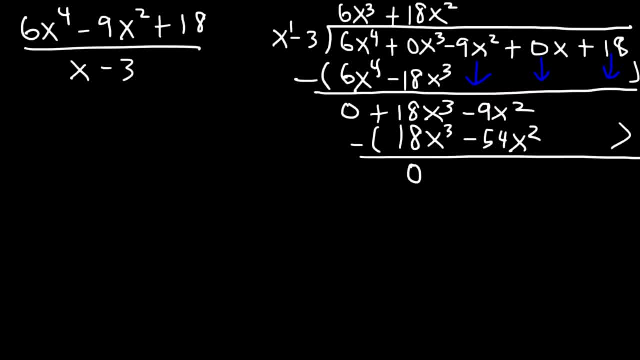 That's 50.. That's something else: 54 minus 9.. That's like 45.. And you could check that with the calculator. So if you type in negative 9 plus 54.. That's positive 45.. Now let's bring down the 0x squared. 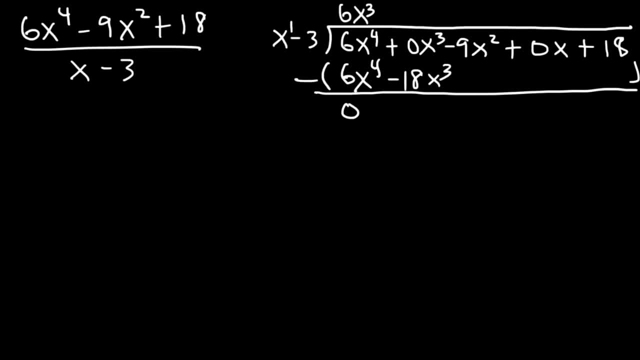 6x to the 4th, minus itself will be 0.. Now 0x cubed minus negative 18x cubed. That's going to be just positive 18x And everything else we could bring it down so we can work on it in the next step. 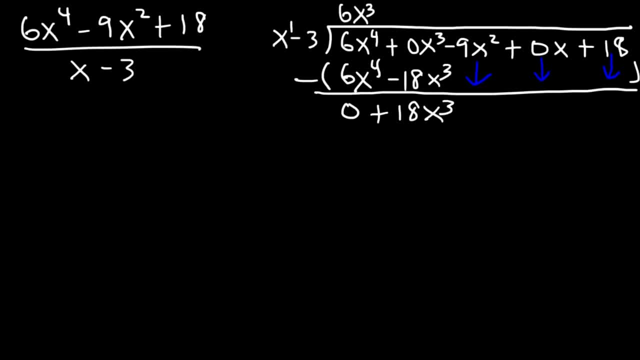 We really don't have to bring down everything. All we need really is just the next term, So we don't have to write the other two terms. We can just focus on these two for now, But if you want to, you can write down the rest. 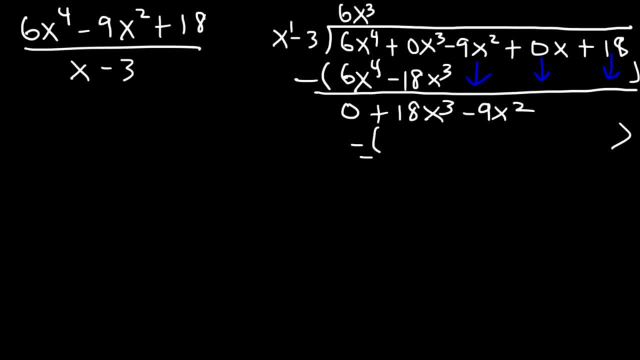 Thanks. Now let's divide 18x cubed by x, So that's going to be 18x squared. And now let's multiply 18x squared times x, That's 18x cubed. And then, if we multiply 18x squared by negative 3, that's negative 54x squared. 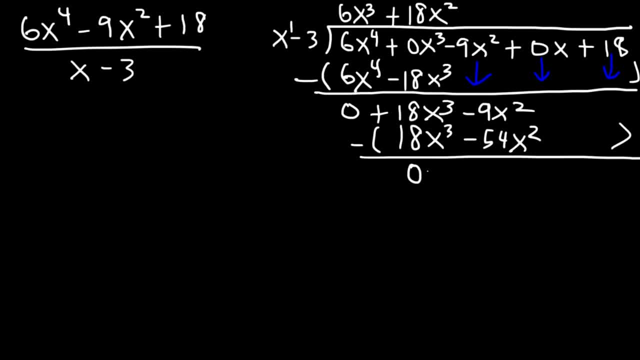 So this is going to be 0. So negative 9 minus negative 54. That's negative 9 plus 54. And 54 minus 9 is basically 65.. I take that back. It's not 65. That's something else. 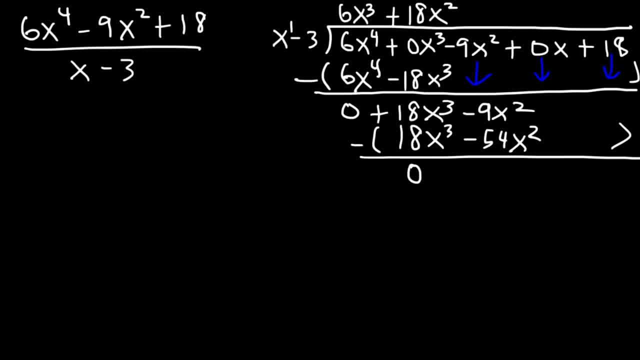 54 minus 9.. That's like 45. And you could check that with the calculator. So if you type in negative 9 plus 54.. That's positive 45.. Now let's bring down the 0x squared, Or I mean the 0x. 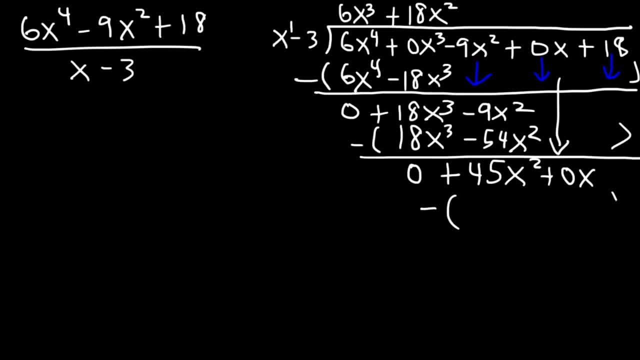 Or I mean the 0x. You know what I mean. So now let's divide 45x squared by x, And so that's going to give us just 45x, And if we multiply 45x by x minus 3.. 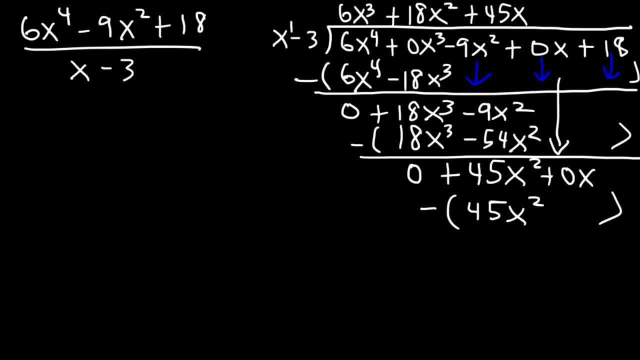 We're going to get 45x squared And 45x times negative 3. That's negative 145x. So this is going to be 0.. And 0 minus negative 145x is positive 145x. Now let's bring down the 18.. 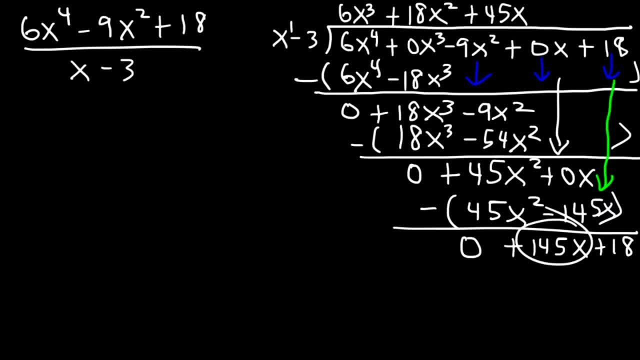 So let's divide 145x. divided by x, That's positive 145.. And 145 times 3.. That's going to be the same thing. And then 145 times negative 3. That's negative 435.. So 18 minus negative 435.. 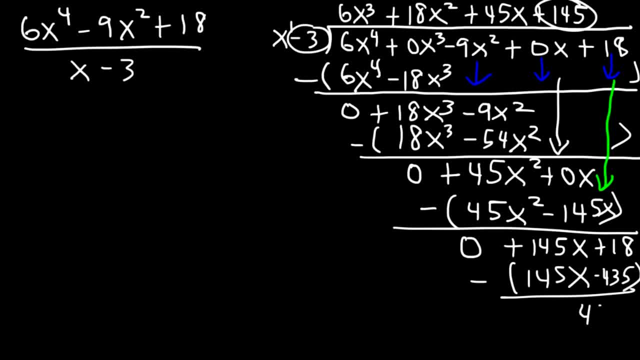 Or 18 plus 435.. That's 453.. So that's the remainder. So this entire expression is equal to 6x cubed plus 18x squared Plus 45x plus 145 plus 453 divided by x minus 3.. 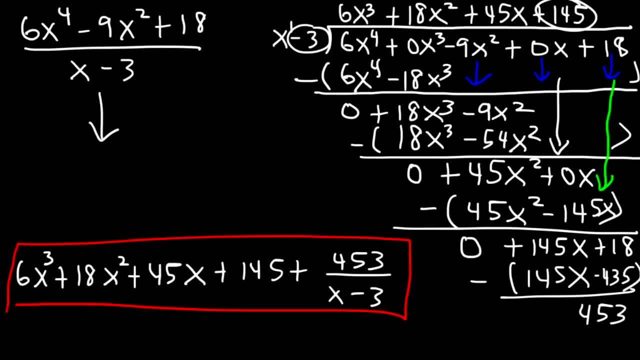 So this is the final answer to the problem. So now you know how to divide polynomials using long division. 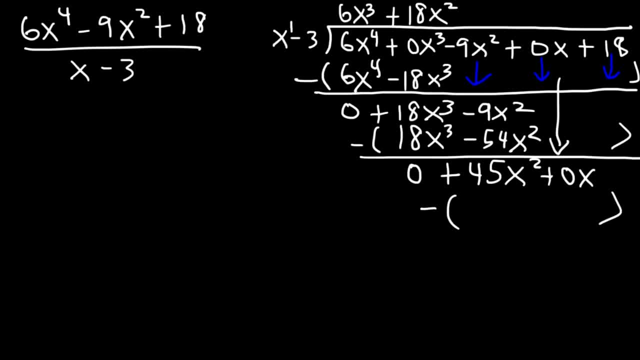 You know what I mean. So now let's divide 45x squared by x, And so that's going to give us just 45x. And if we multiply 45x by x minus 3. We're going to get 45x squared. 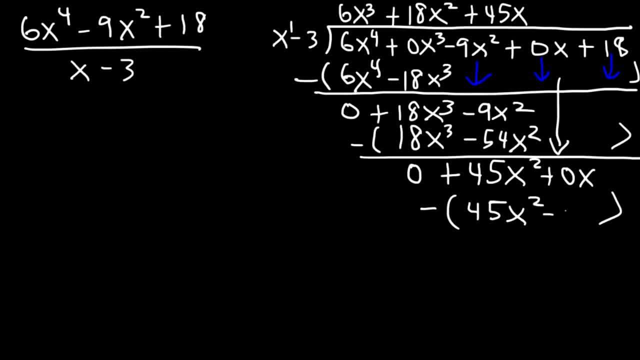 And 45x times negative 3. That's 45x squared Times negative 3. That's negative 145x. So this is going to be 0.. And 0 minus negative 145x is positive 145x.